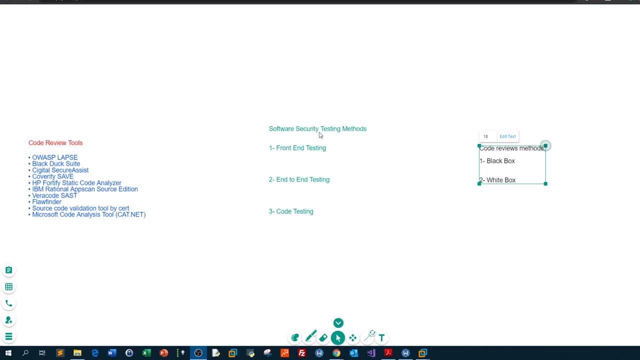 testing guys. We know where you have a piece of software that's being developed, programmed, and then this piece of software will be deployed and implemented to be sold to the customers as a solution. So every program, you see every bit of software, whether it's free, open source. 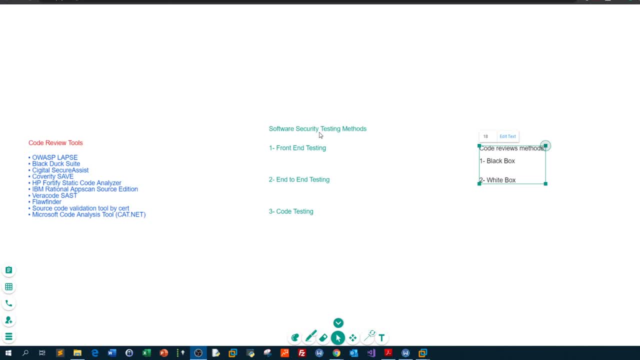 commercial. it has gone through many stages To be from the design, the development, the implementation, testing, all the way to the production and release to the public. So software security testing guys is an approach to just put security as a concern while developing. 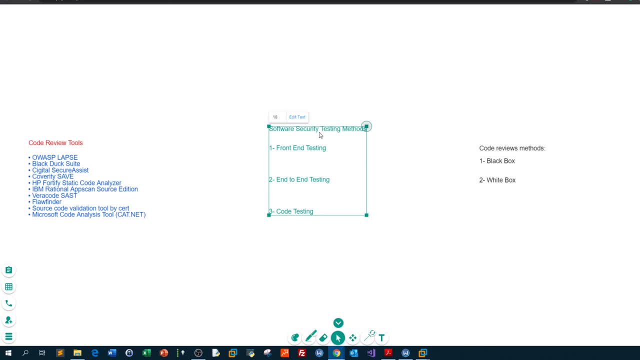 softwares or programs. Software security testing is all about making sure that the program or the software we are developing is secure enough to prevent flaws, exploitations and any kind of errors that would come along the way while the software is being used by customers or clients. 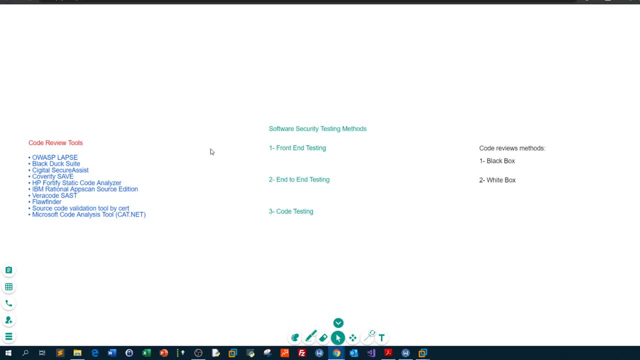 It's embarrassing, you know. So, software security testing, guys, in a nutshell, there are three methods for testing a software for security. We have the front-end testing, we have the end-to-end testing and we have the code testing. So, in a nutshell, guys, front-end testing, it is testing the software. 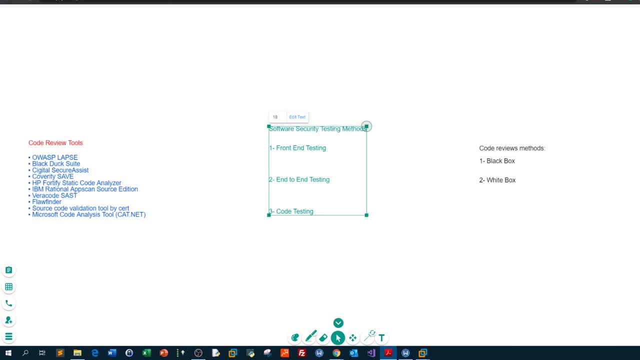 okay, It's all about testing the software against. you know from the front end Like you are the clients. you have bought the software and you are now experiencing the use of that software. Consider, for example, a testing case like input validation, SQL injection, cross-site scripting, operational. 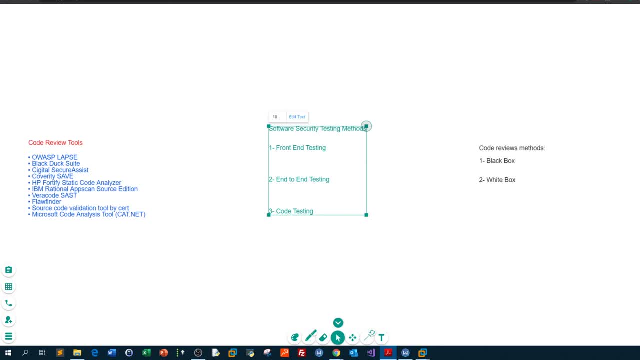 testing, authentication mechanism of an application. So these, all these kind of tests are carried on or, sorry, are implemented, are done from the front end of the program. okay, Like any user- whether the user is malicious or an actual client- is experiencing and trying to use the software from 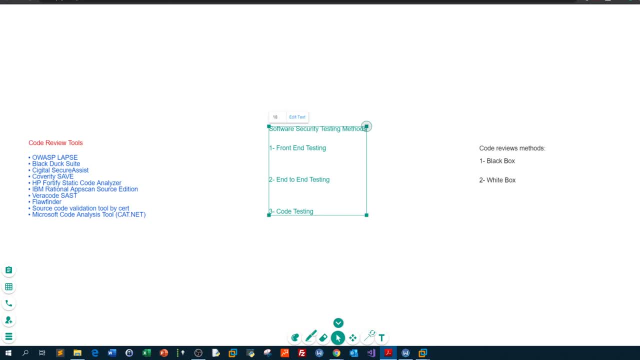 the front end. So you are doing the same, okay, as a developer or as a security consultant when you are testing the software from the front end. So basically this type of testing guys- you know it's focused on some aspect of the security life- 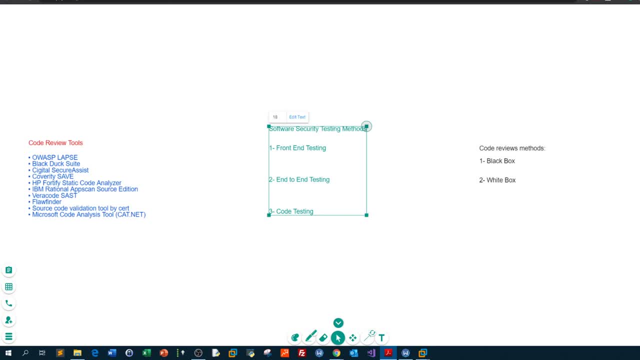 cycle, but it's not comprehensive. okay, Now the end-to-end testing over here, guys. it is the most effective type of software security testing in which complete security assessment is carried, performed to cover a wide range of security controls, like the aforementioned testing on the front end. In addition, we review the source code, we review security misconfiguration, we review 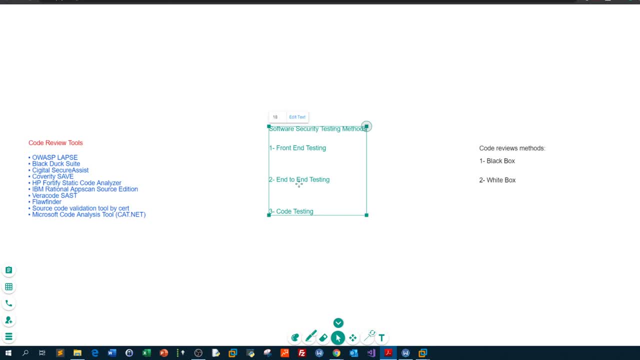 the security equation. we review the data that is running behind the software. we try to test the security database, the records, the administration, just you know, a comprehensive test from the front end to the back end. Now the code testing guys. code testing is well, it is kind. 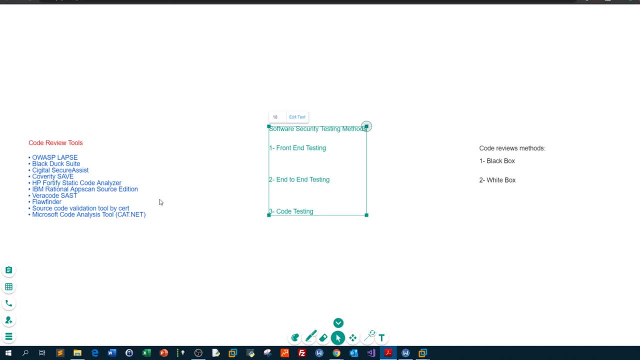 of complete code review. So, for example, you got like thousands of thousands of lines of code for your program. code testing is all about reviewing this. okay, video guys, we're gonna go through code testing. okay, so how we can achieve code testing if we? 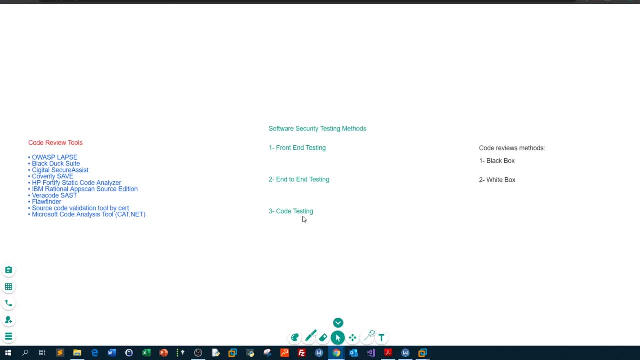 have like thousands, of thousands of lines of code. how are you gonna test this manually? well, we have methods to test code guys, basically, as you can see here. uh, okay, so here, code review tools. we have many tools guys to review security code. um, one of these tools guys, as you can see which. 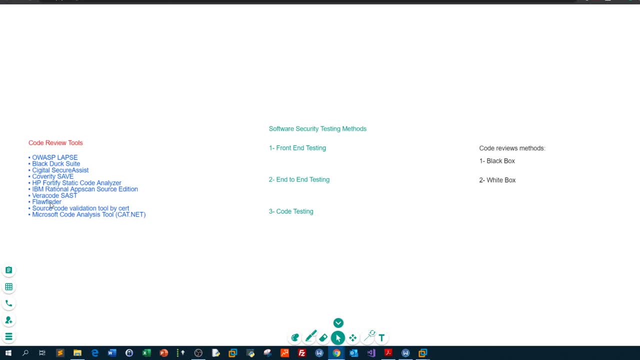 we're gonna use in this video is a flow finder. flow finder. we're gonna use, uh, this tool, guys, and try it on a sample code to test, uh the code for vulnerabilities, so you don't need to go through thousands of thousands of lines of the codes to see whether the code is vulnerable or like. 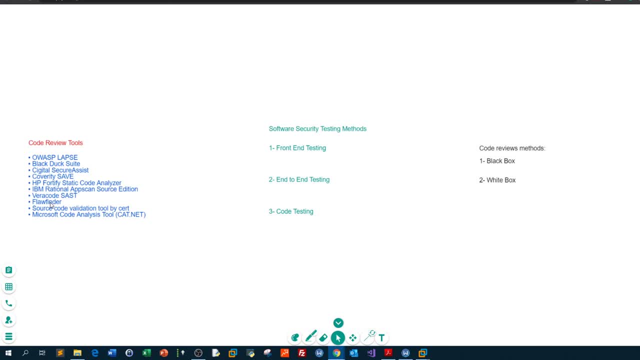 whenever, like buffer overflow, exception handling, um, or, let's say, sql injection or crystal scripting or what whatever. so all you got to do is to run one of these tools on your code and the code- oh sorry, the tool will try to identify the lines of code that would raise a vulnerability for your 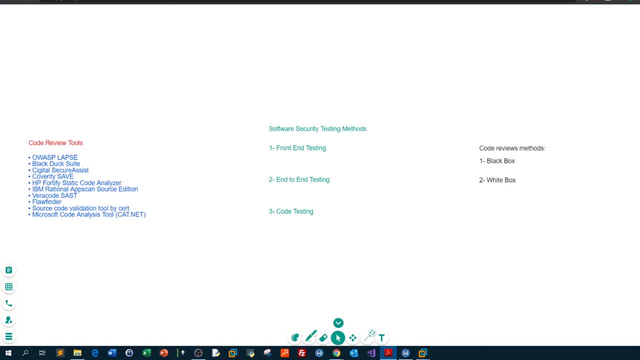 code. i'm not saying that using tools is a comprehensive view for your code. you're just trying to do things like that with a lot of speed, which is one of the reasons that i'm gonna do this: learning the code, testing examples, which is a comprehensive view for your code. you just 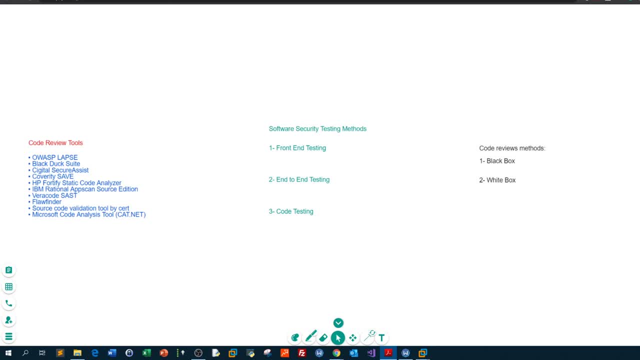 got to use the tools as a first line or early in your testing, okay, and then, when the tool identifies the lines of code that are vulnerable, you're going to go through all of these lines manually, okay, and you're going to identify how to fix the errors, how to fix the vulnerabilities. 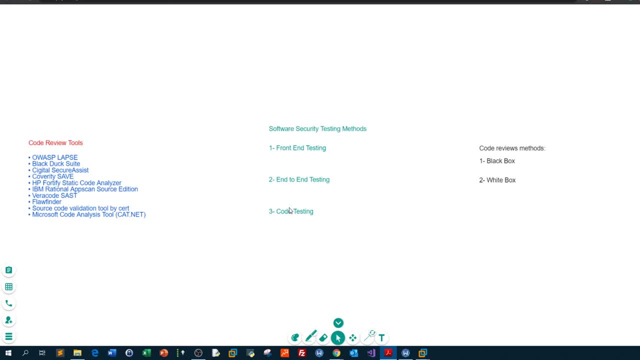 of course, if you, the other the other time of testing is to go through the code line of codes manually, you cannot achieve this alone. you're going to have you need to have a second option or a second security professional or other security professional who stands by your side. 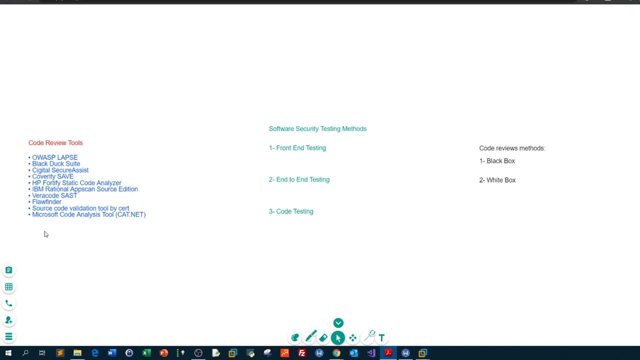 to review the code manually. so we can review codes using the tools. okay, and we can review the codes manually. so, guys, reviewing codes using the tools is called the black box method. okay, so black box is reviewing your code using the automated tools. you, the white box, is reviewing the code manual with your peer security professional. 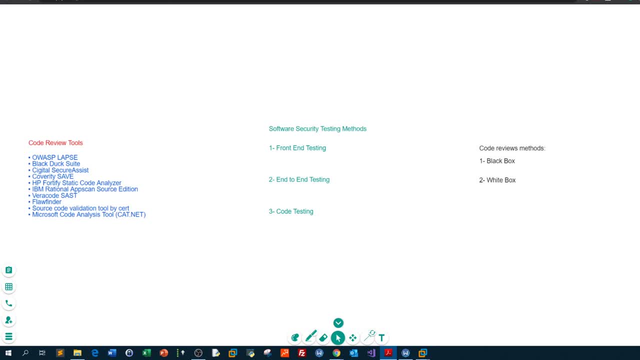 okay, now let's jump in to cali linux, okay guys, and see how we can use flow finder to examine the vulnerable code. now let me switch my uh display, you, i think. i think i'm having difficulties showing the other display here, but let me try to delete this from here. remove, okay now. 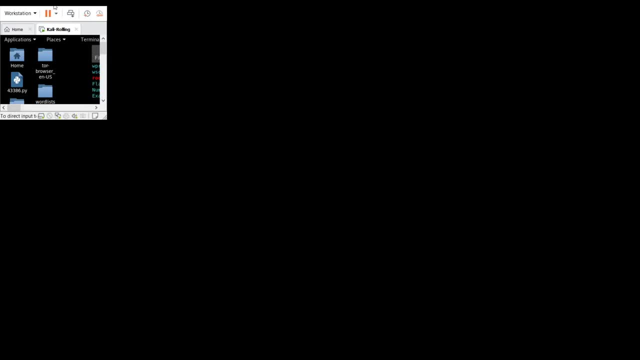 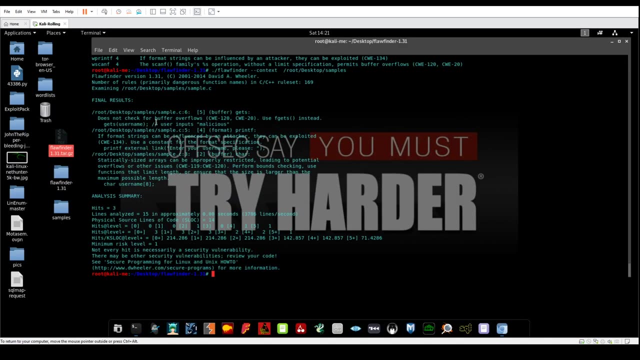 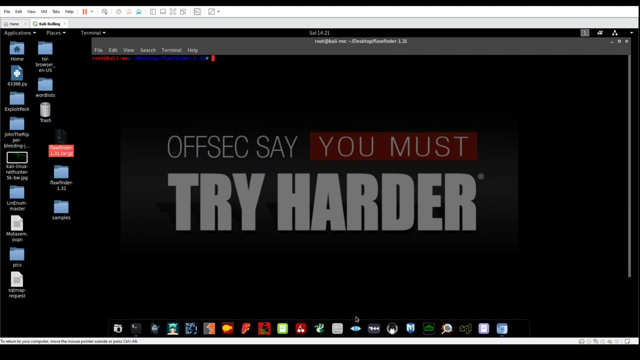 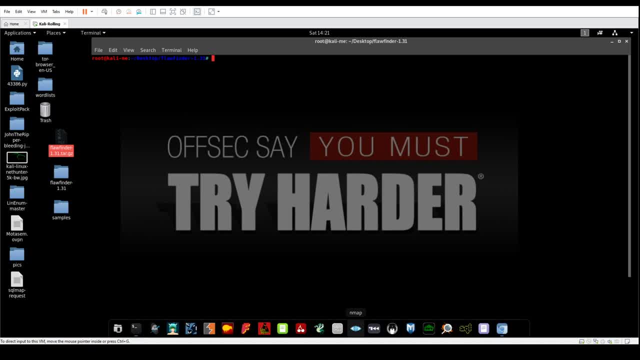 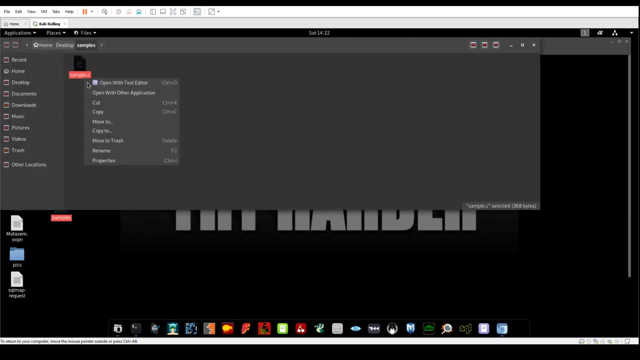 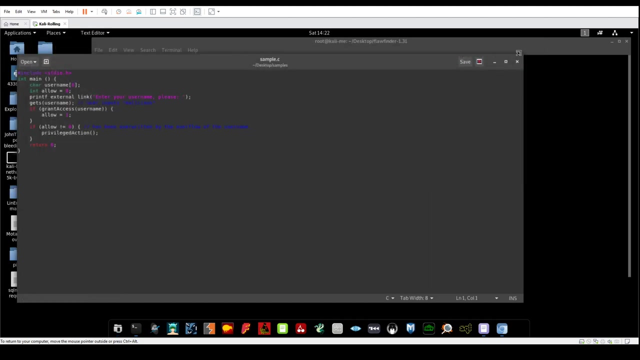 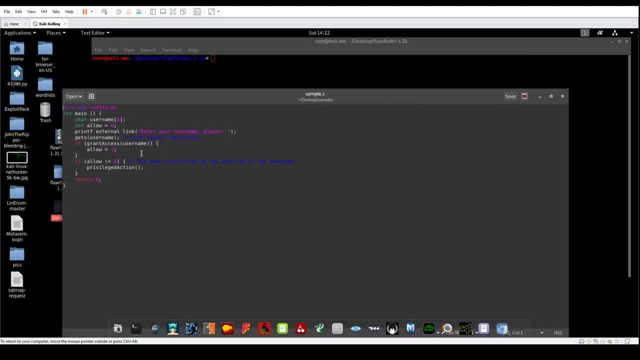 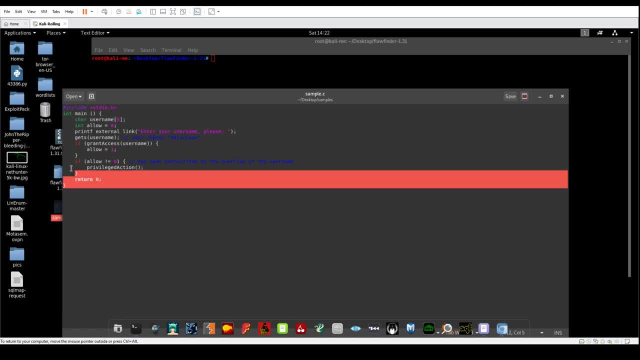 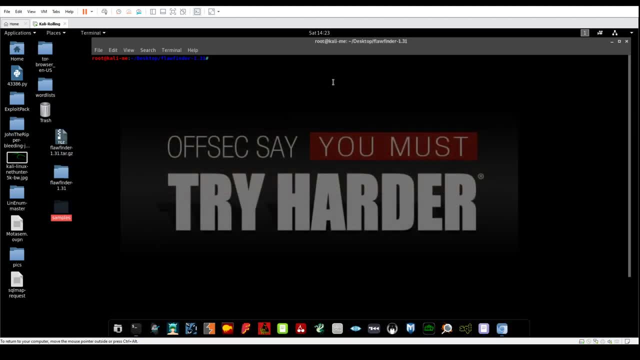 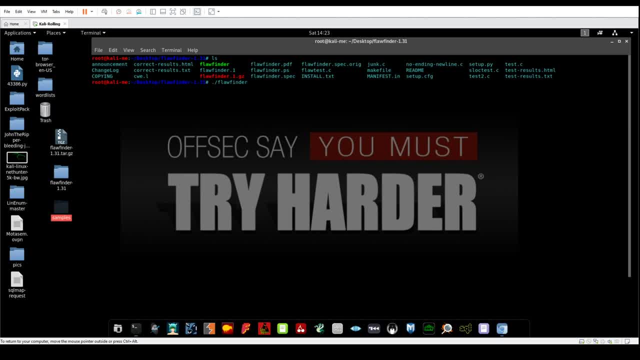 our sample code or the target code that's about to be tested, we feed that to the flow finder. so, basically, we type root desktop samples and if you have more than one C code, all you got to do, guys, is to place this define inside the folder okay, in which? all of your scripts, all of your files for cleaning whatnot something occur in your string groups and we start my Strings for you guys. and once everything fields stop wandering, you know change the status and you know why. nobody starts avoiding issues. right now, kind of like right now. 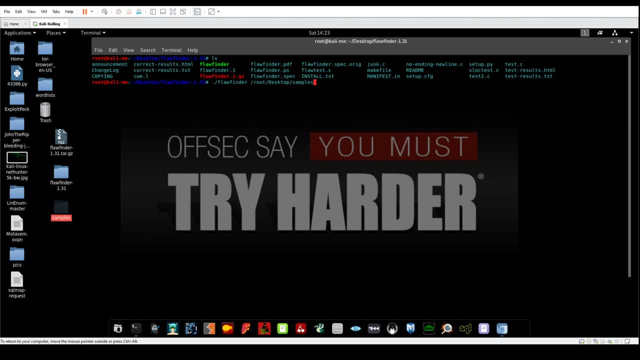 your file that are supposed to be tested. okay, you place them in that place, in that directory, in that folder, and the flow finder will test all of these scripts, all these codes. but it's better when you are testing for production, this one by one, it's better for you to examine the results more thoroughly and 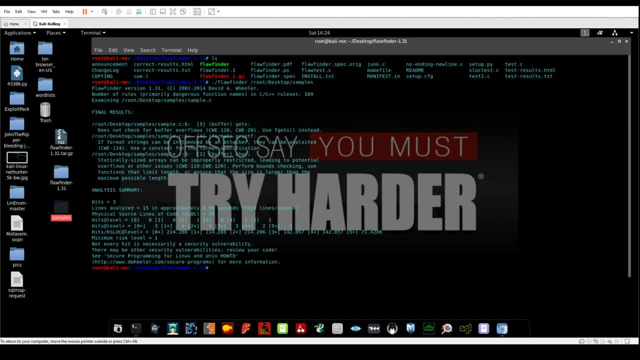 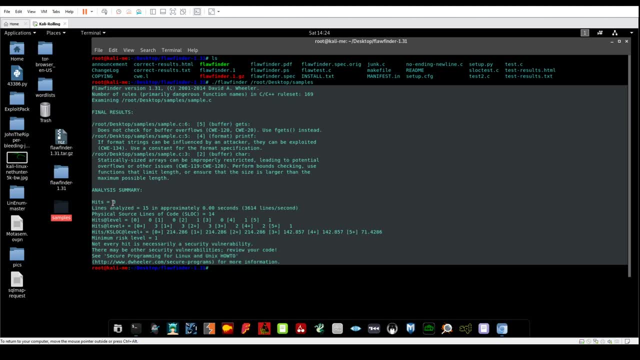 deeply so hit, enter and receive the results. it's very fast, as you can see here. analysis summary. it says hits equal three. so when we say, when we say hits equal three, it means that we have three instances in the code that may have potential vulnerabilities to be. 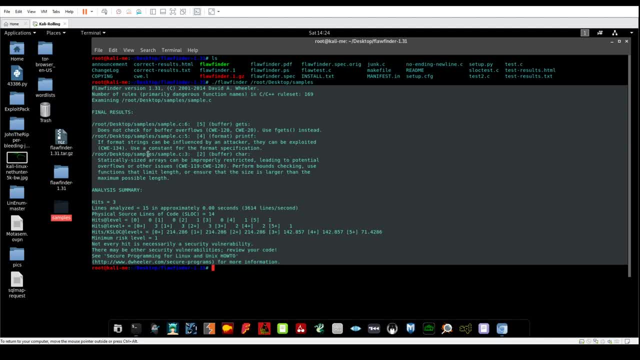 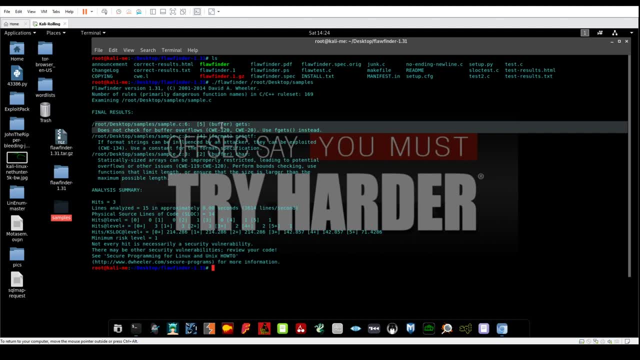 exploited guys. so let's look at this. these three hits the first one. so it says in line five: okay, we have a buffer, okay, and it says your buffer or your or the function you you have used, okay, it doesn't check her buffer over flows, so you: 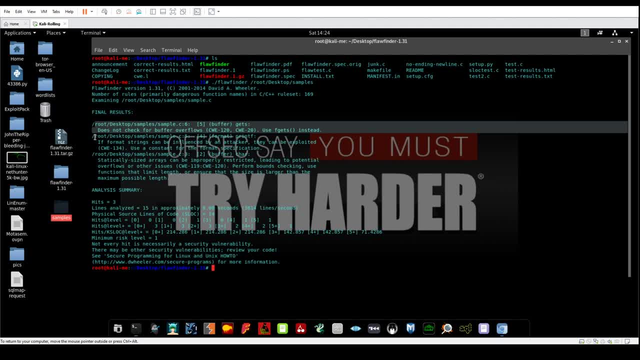 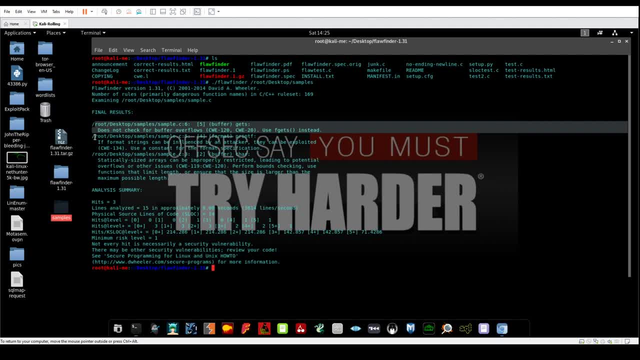 library parameter whatsoever. it lists you the line, the number of line- okay- and it lists to you what's the wrong, what's wrong with this, and it tells you what to use instead. okay, so we can. we can display more thorough results by examining what what's, what's the exact vulnerability in every line of code and how we can fix us. 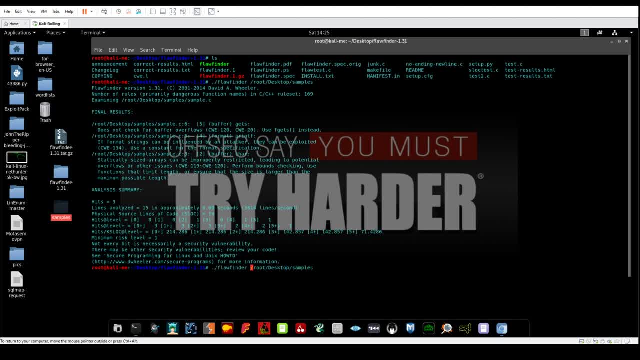 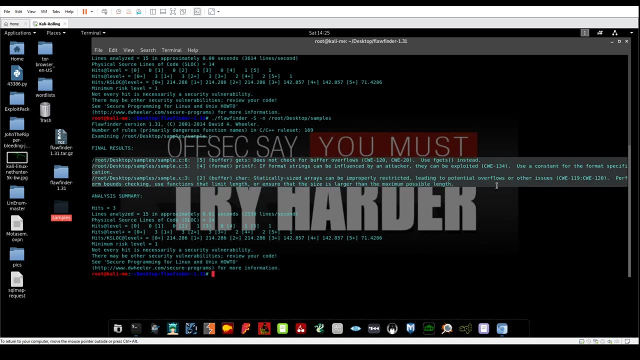 we fix that so we can run the same command but instead we can run context or not. uh, s the switch s and n. all right, so let's go ahead through our results. as you can see here, it says in defy samplec, line six, we have buffer gets and it says: doesn't check for buffer over. 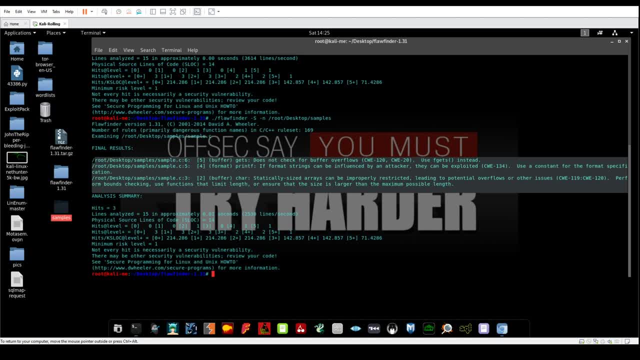 loads. use f gets instead. okay, i got this. the second one. it says you have used printf and if format strings can be influenced by an attacker, they can be exploited. use constant for the format specification. so for every line. so we have what you have to do, guys, is you go to the code? 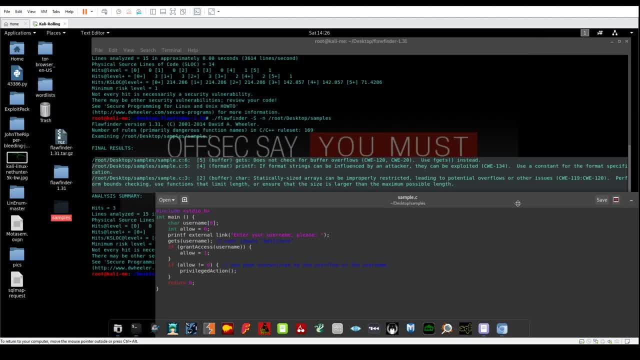 and let's see here. so set line six, one, two, three, four, five, six. so instead of gets, i use def gets, for example, as per the recommendation. and the second one, it says if former strings can be influenced, uh, use a constant for the format specification in line number five.